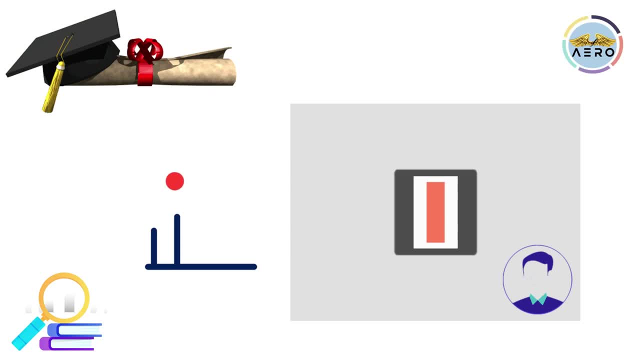 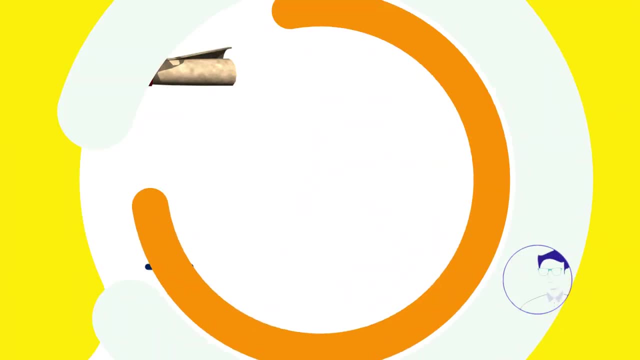 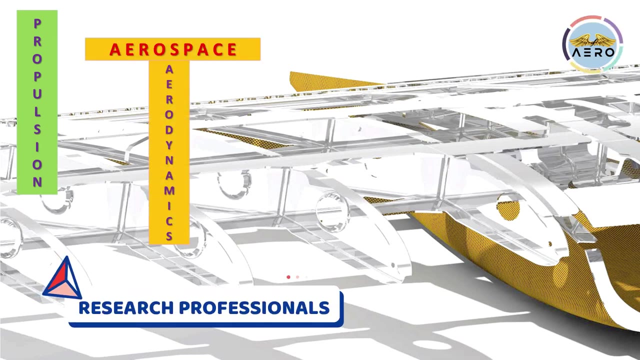 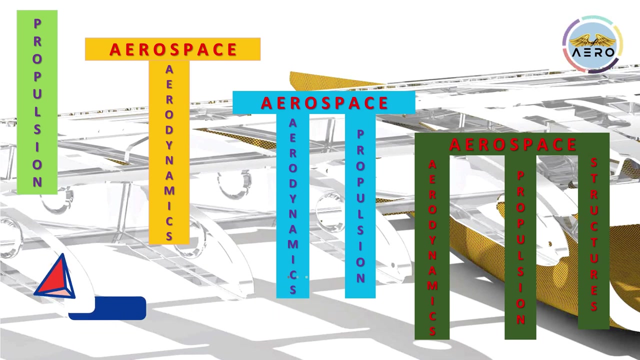 This video is made completely based on suggestions from experts and from the market survey. Before proceeding to the aerospace research topic, you must understand the sensible professionals like I-shaped professional, T-shaped professional, Pi and M-shaped professional. So I-shaped professionals are having a lot of experience. 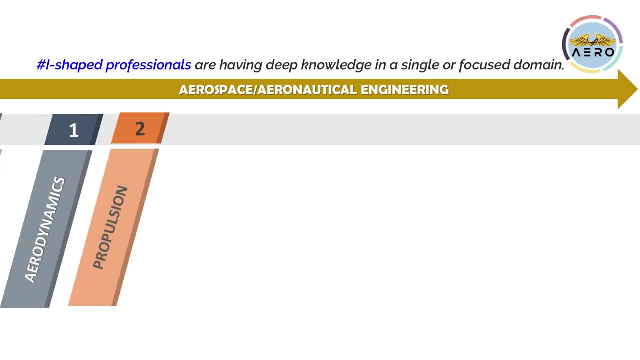 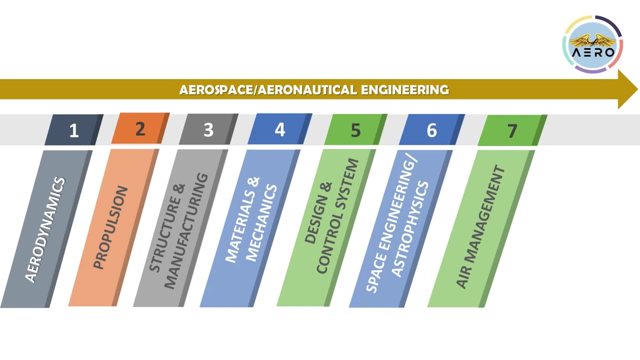 They have deep knowledge in a single or focused domain. For aerospace, focused domains like aerodynamics, propulsion, structures and manufacturing, materials and mechanics, design and control systems, space engineering or astrodynamics, then aviation management or aerospace medicines. Each individuals are considered. 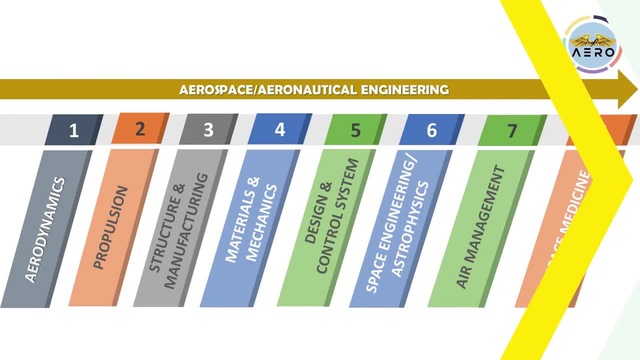 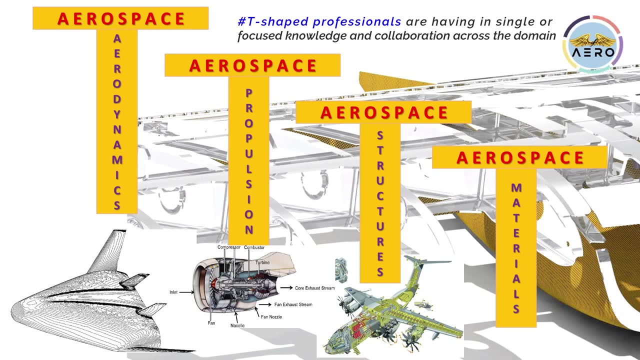 To be as I-shaped professionals, So T-shaped professionals means single or focused knowledge and collaboration across the domain, For example, how the applications of aerodynamics is widely implemented in supersonic, subsonic or even hypersonic field in the aerospace domain. 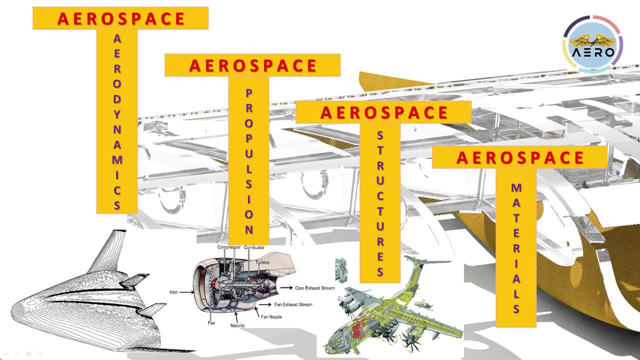 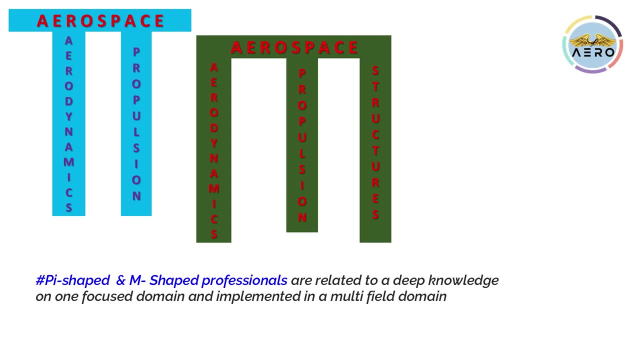 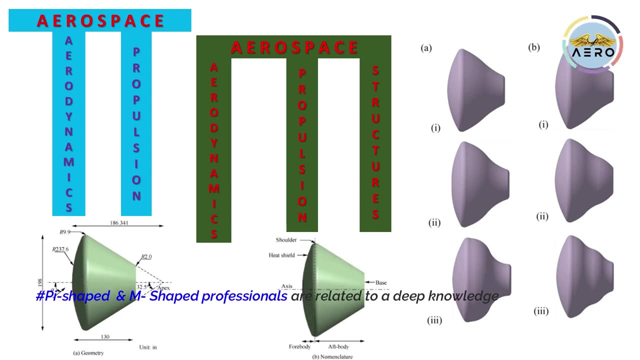 Now talking about Pi and M-shaped professionals Are qualified, Related to a deep knowledge, or in one focused domain, or implemented in multi-field domain. Moreover, it's, like you know, compiling a combo of aerothermodynamics structures, controls into one research topic. 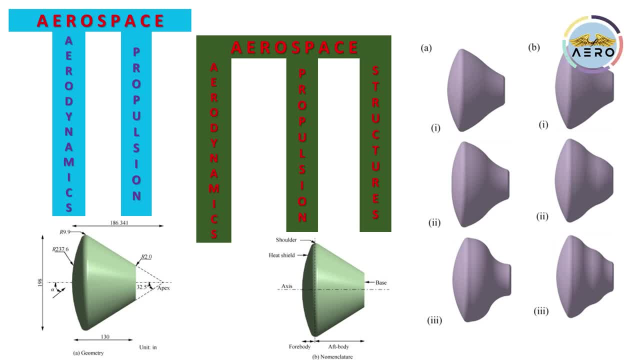 For an example, aerodynamics and aerothermodynamics of reentry vehicle. In this you must have a knowledge of more than one domain Like aerodynamics as well as a propulsion is considered. So it will be considered as a Pi-shaped professional. 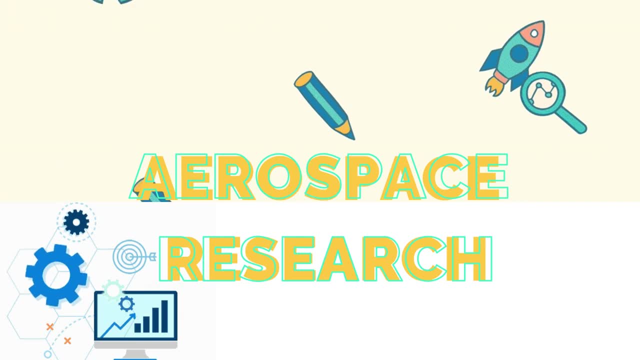 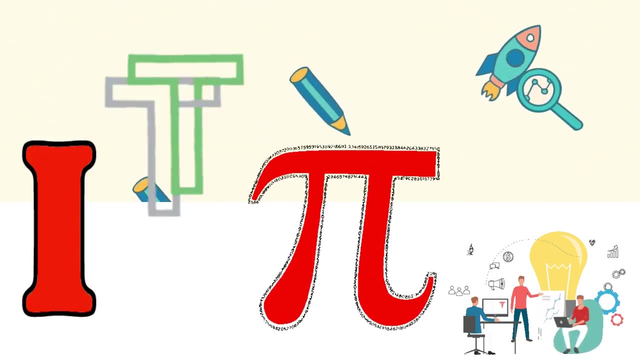 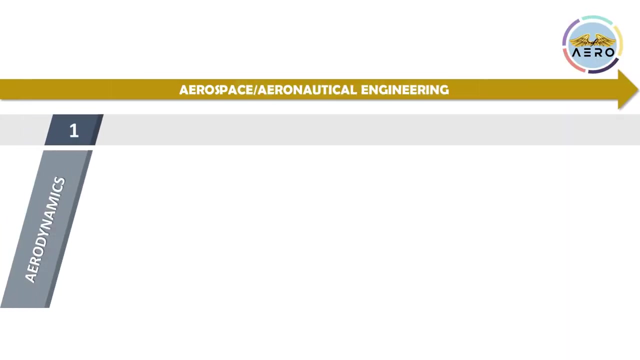 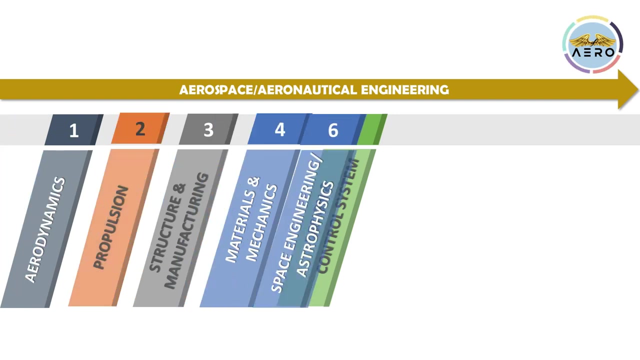 Today I will discuss a possible aerospace research topic or the thrust areas based on I, T, Pi and M-shaped professionals of each aerospace domain, Like aerodynamics, propulsion, structure and manufacturing, Materials and mechanics, Design and control, Space engineering. 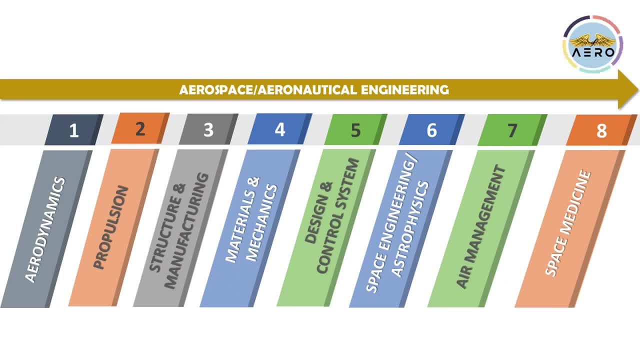 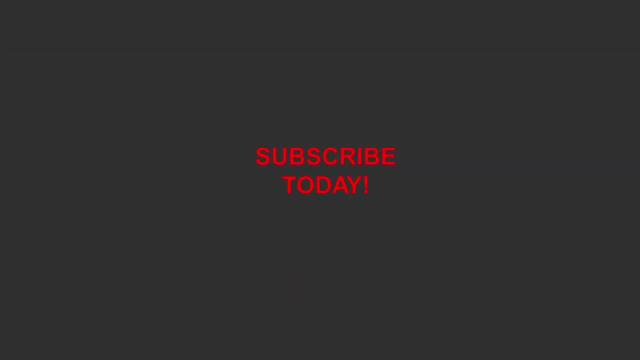 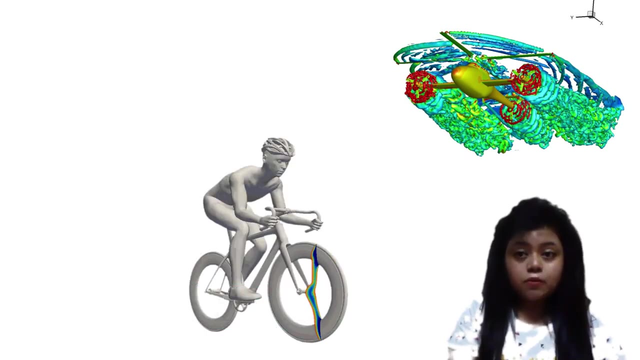 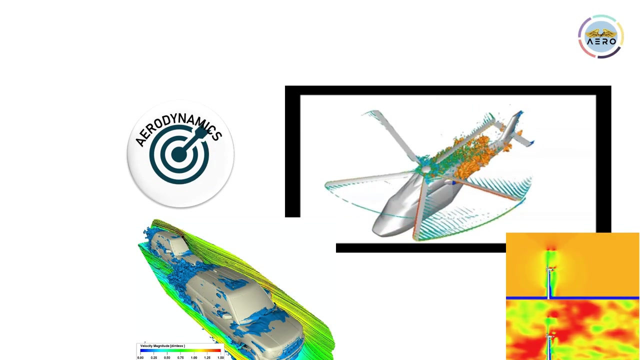 Aviation management And aerospace medicines. So let's start with applied aerodynamics, Which covers a broad range of research topic, both in aerospace domain As well as multi-field domain. Any research work on aerodynamics evaluated either through scientific computing, through CFD and numerical methods, or by means of experimental investigation. 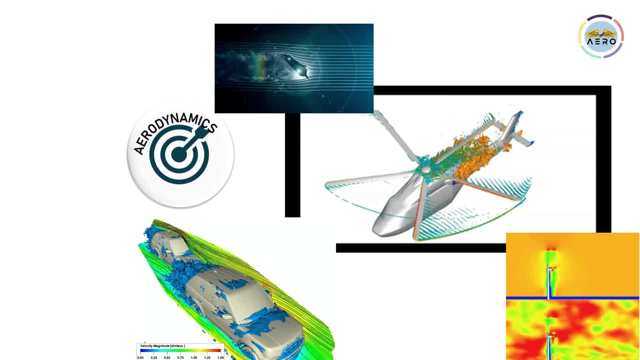 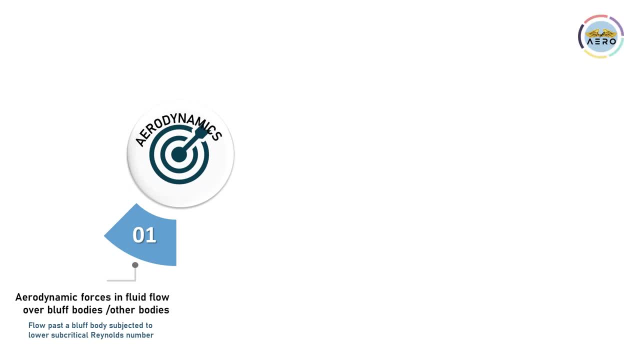 So the most possible topics are Aerodynamic forces in fluid flow over a rough body or any other body. Second comes unsteady flow Or transitions and the turbulence or the vortex dynamics. So here you can see few examples like numerical investigation of cavitation vortex dynamics in unsteady cavity flow with a shock wave propagation. 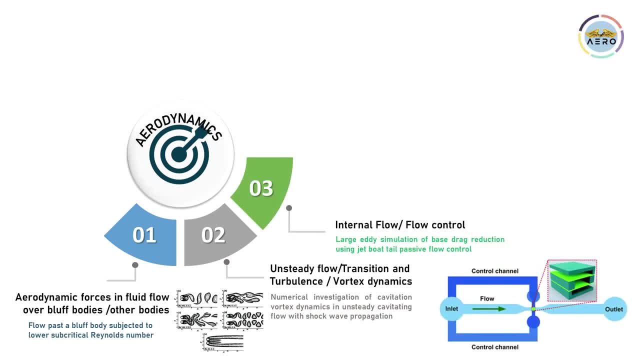 Then internal flow or a flow control. It can be either active or passive control of jets, Like a large area simulation of a base track reduction using jet boat tail. passive flow control, Then aerodynamic shape optimizations. This is widely used in aerospace field. 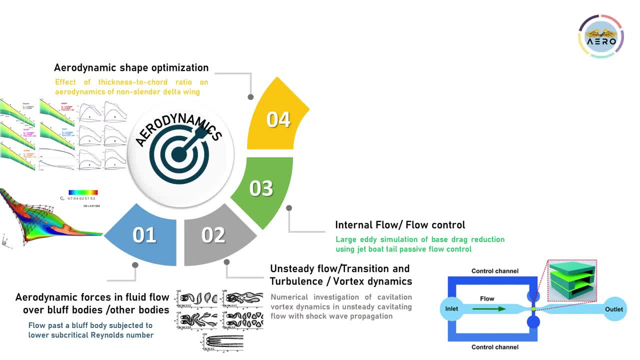 Like an example effect of thickness to chord ratio on aerodynamics of non-slender delta wing. There are lot many research you can do on the various configurations of the delta wing too. Then experimental fluid mechanics or wing channel techniques in subsonic or supersonic or even hypersonic field. 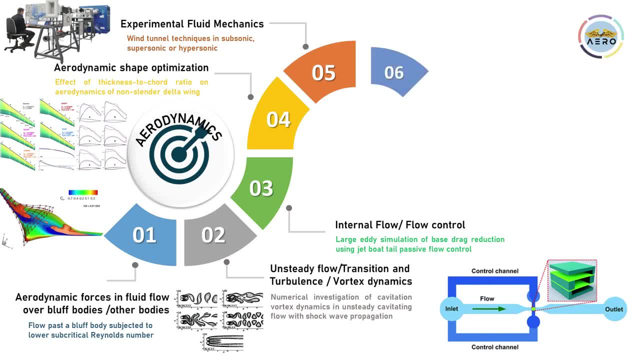 Then helicopter aerodynamics. In helicopter aerodynamics you can majorly do a research on rotor blade aerodynamics, Then separately research can be done on especially foreign blade aerodynamics, Then coming to an hypersonic aerodynamics. At present a much work is going on on this particular field. 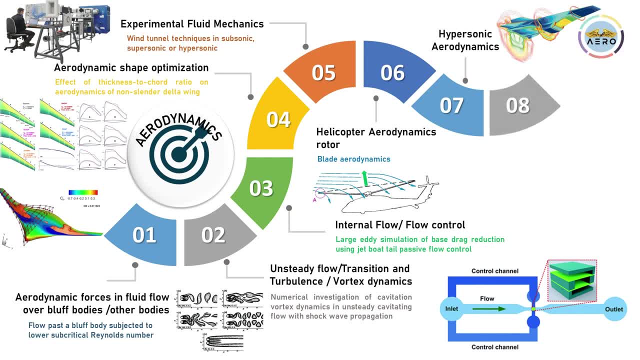 Even a missile aerodynamics, Like an example, investigation of acceleration effects on missile aerodynamics using computational fluid dynamics. There are ample of research going on Such amazing topic also you can pick, like effects of rainfall on an aircraft aerodynamics Or the cross-section. 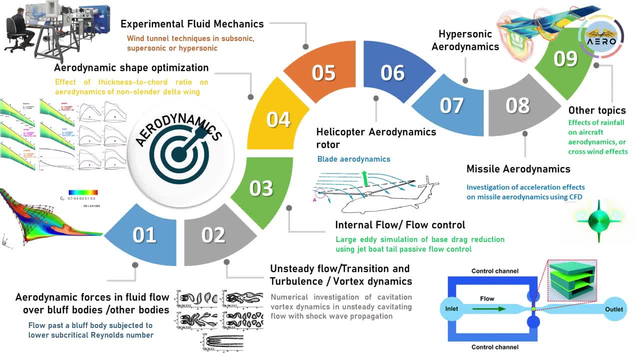 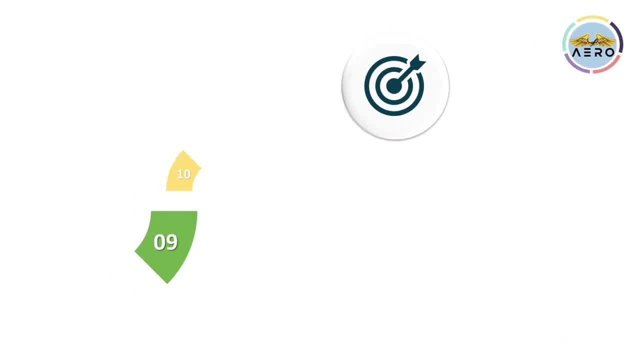 Or the cross-wind effects. Now I will tell you some of the aircraft aerodynamic concepts is applicable in other fields, Like aerodynamics in wind powered device, Like comparison of the power lift or the drag coefficients in the wind turbine blades Or other the aerodynamic characteristics varying the airfoil. 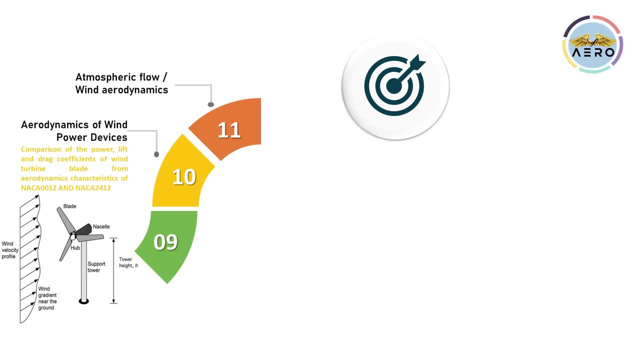 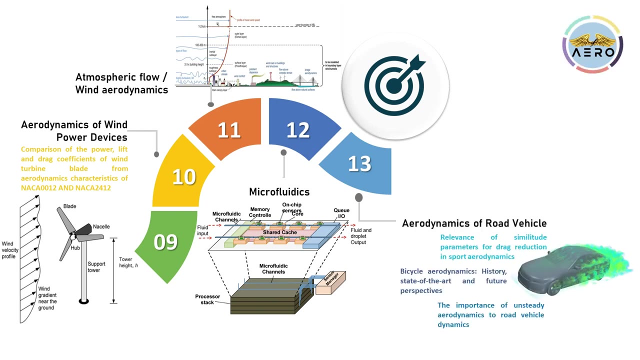 So then, talking about the atmospheric flow or the wind aerodynamics, Again, some more precise research can be done on microfluids, Then aerodynamics of road vehicle, like sports car, or even high speed train, bicycle. Actually, this is actually industrial applications of aerodynamics. 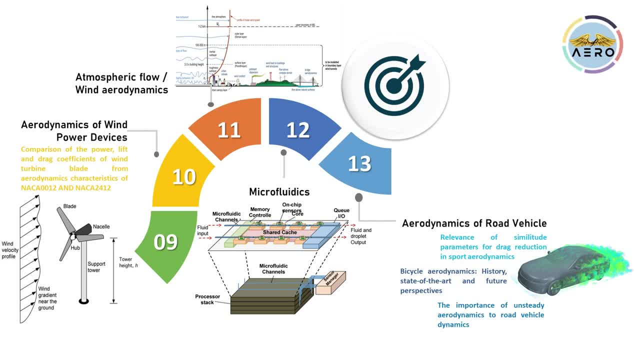 There are lot many research going on, Like relevance of simulated parameters of drag reduction in sports aerodynamics Or even bicycle aerodynamics, Even the importance of unsteady aerodynamics, Unsteady aerodynamics to the vehicle dynamics. There are lot many industrial applications are also going on. 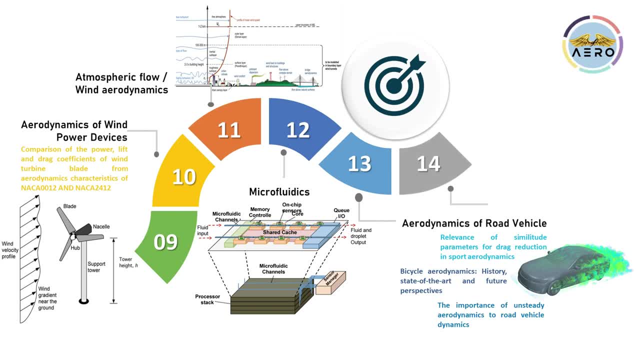 Then even marine vehicle dynamics, Building or a bridge dynamics. You might have heard about the Takonoma bridge incidents. That is also further. it has been studied about the bridge dynamics And now we have made a better advancement in the research. All individual topics are high shape, professional. 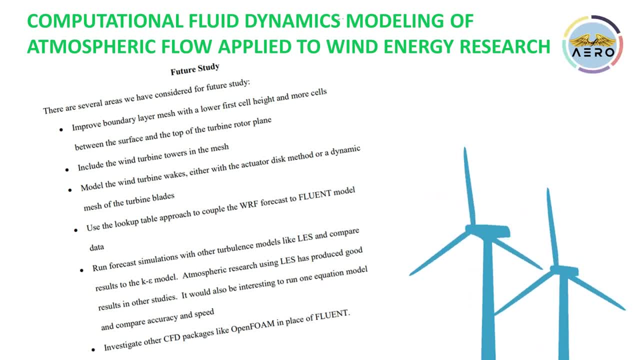 Suppose, any person combinedly working on blade dynamics Along with the atmospheric flow and the experimental fluid mechanics Will probably fall under the T shape professional. In upcoming talks I will be giving you an example Of how the research work can be compiled with other domains. 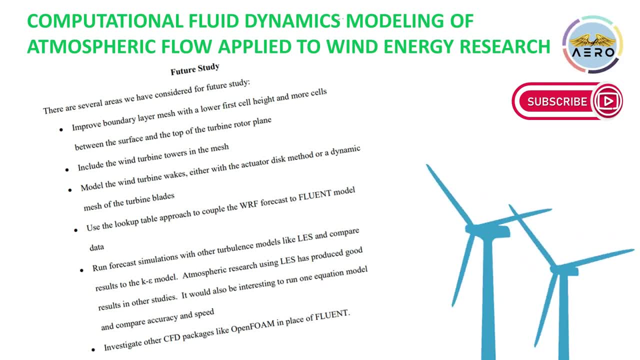 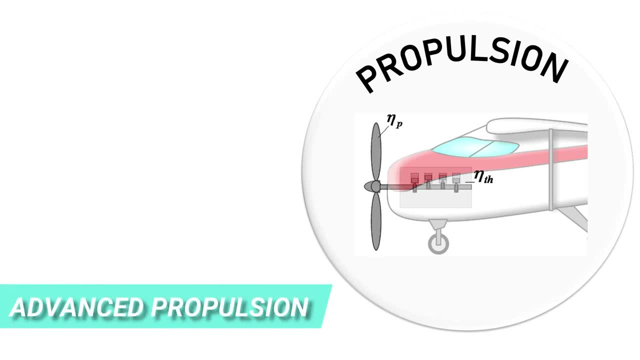 Like propulsion structure and so on. So stay tuned till the end of the video. Next I will move to the propulsion research topic. Sometimes it is also called as thermal and propulsion core, So are as follows: In air breathing propulsion. 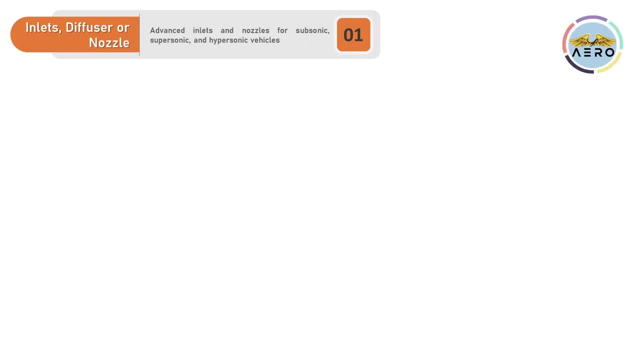 Now work on inlets, diffusers or nozzle for a various flight speed, Even advanced inlets and nozzles for subsonic, supersonic and hypersonic vehicles. You can work on Even combustion fuel flow reactions. It can also extend to a fire dynamics. 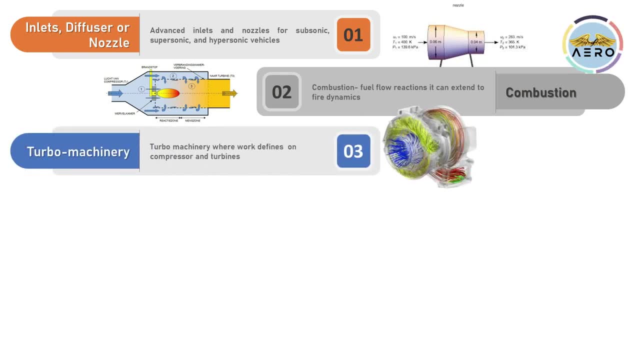 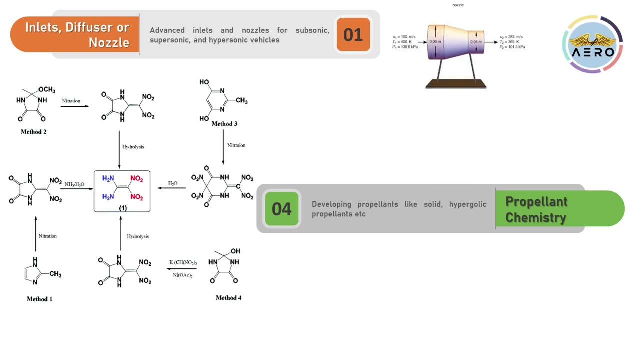 Right. Then even turbo machinery, Where work defines on the compressor and the turbine. If I talk about the rocket propulsion Now, there are lot many work going on in developing propellants Like solid hypergolic, monogolic propellants. 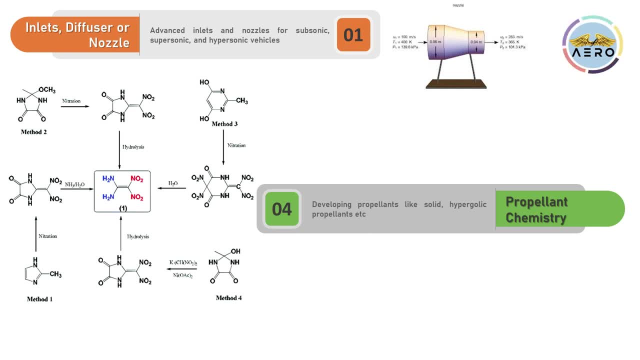 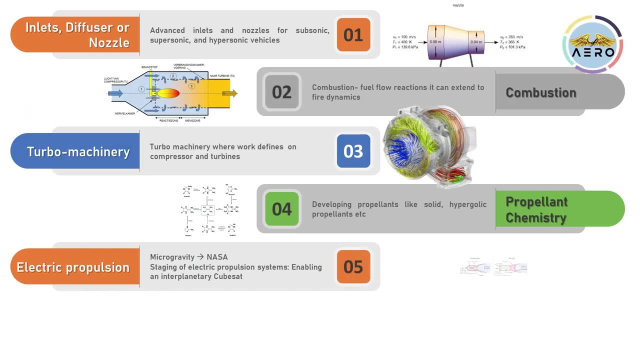 Sometimes you can also like It is also known as propellant chemistry. You can do a research on it. Then, electric propulsion: Now talking about electrical propulsion. Electric propulsion Now. microgravity, where the NASA is experimentally working on. 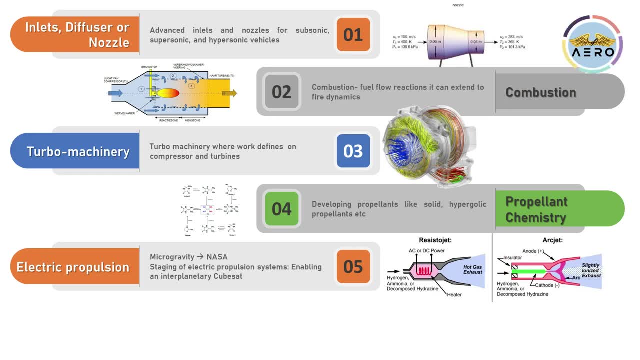 Like even CubeSat, All of you might be knowing. Even that is a part of electric propulsion. So then, talking about thrust victory, Either a primary or the secondary. It is widely used in the rocket propulsion or in the space. Either we can talk about the rocket or the spacecraft. 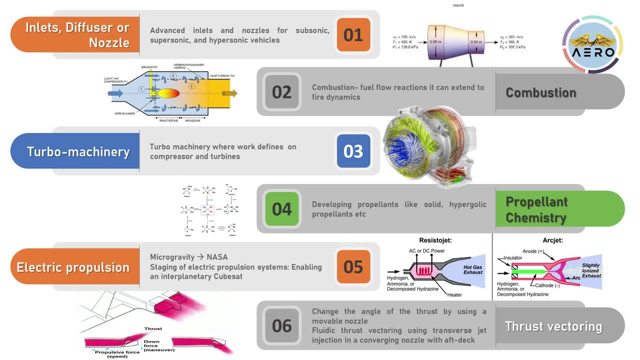 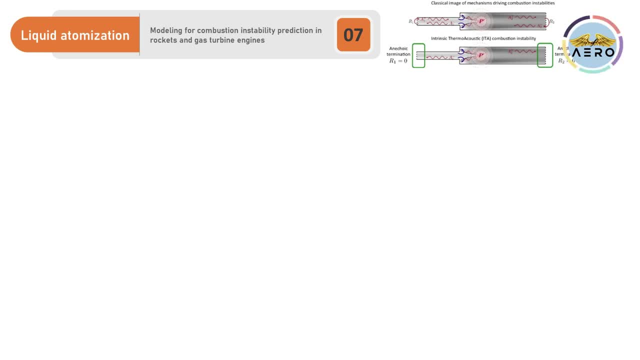 Then coming as the liquid atomization and spray combustion. This is also play a very important role. Similarly, you can also work on the modeling For the combustion instability predictions in rocket or even the gas turbine. Then heat and mass transfer. 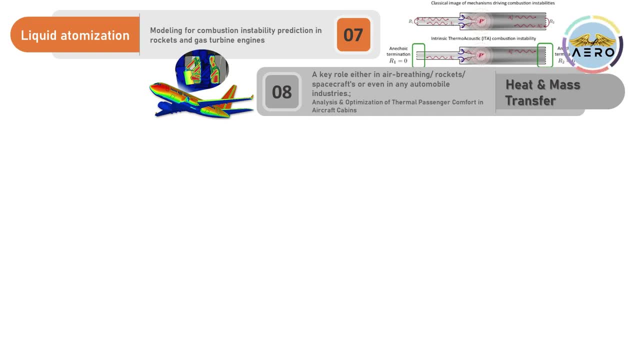 Play is a key role, either in air breathing or rockets or the spacecraft, Or even in automobile. in vastness, Then, cooling techniques. When it is we are talking upper thermal, There must be some kind of cooling techniques. It is very important. 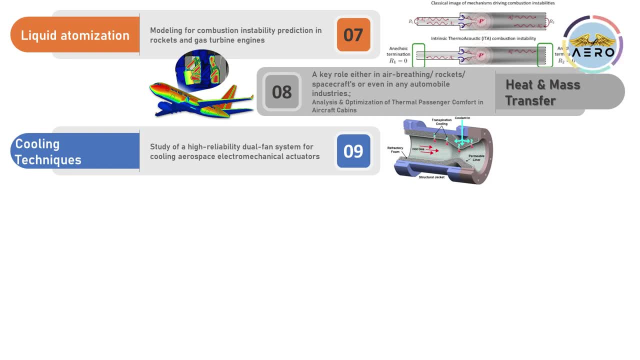 This also play a key role And also cooling, directly or indirectly, plays a key role in efficiency. So another work you can do is a cryogenic application. There is a wide, wide, wide opportunities to work on cryogenic applications, Either in the engine or the fluid. 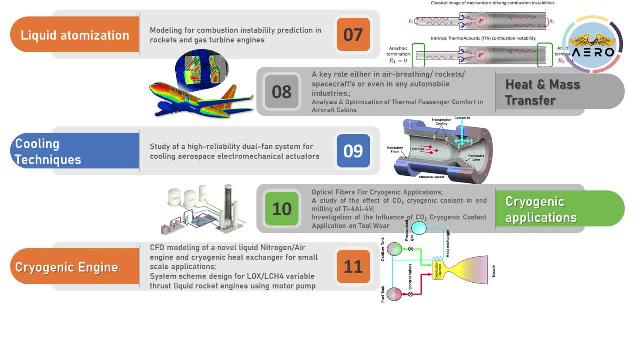 You can work on by various means. Then another very special topic is a bio-inspired propulsion Like a bio-fuel. Basically it is a pie-shaped profession. You can talk where one need to have an idea about the vegetable oils, Or even aviation fuel and its composition. 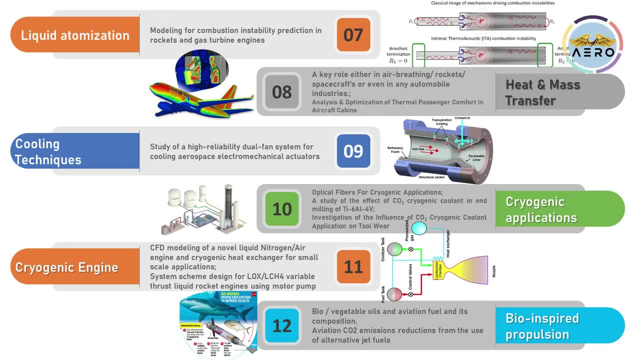 So there are lot many research going on since 2005,. I think Yeah. So even some of the aviation industries are going on. You can see an example: Aviation CO2 emission reductions from use of alternative jet fuels. There are lot many research you can do on it. 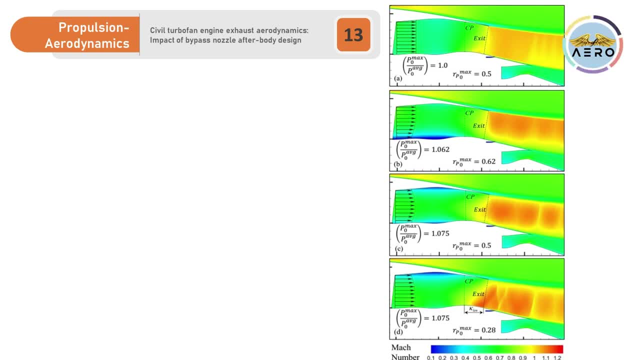 But there are certain research topic Okay, Where the movement of air is crucial to both aerodynamic vehicles and the efficient engine, That it can't be isolated from aerodynamics and propulsion, Like some research has undertaken on civil turbofan engine exhaust aerodynamics. 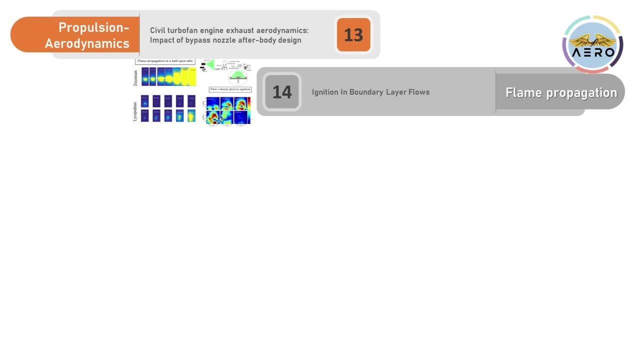 There are lot many research is going on. Similarly, you can also take one of them, Then flint propagation and ignitions in boundary layer flow, Then multi-phases and the reactions to form in a complicated system, Either in the form of gas liquid or the gas solid or the liquid solid interface. 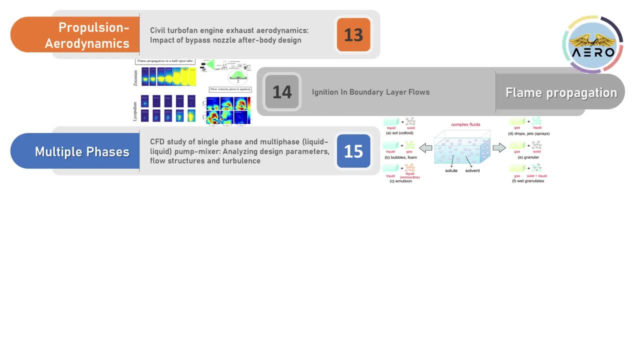 There are lot many also projects are going on On the CFD study of a single phase or the multi-phase pump mixture. Or even, if you talk about this rocket engine, When the cooling system is done in the cryogenic rocket engine. Okay. 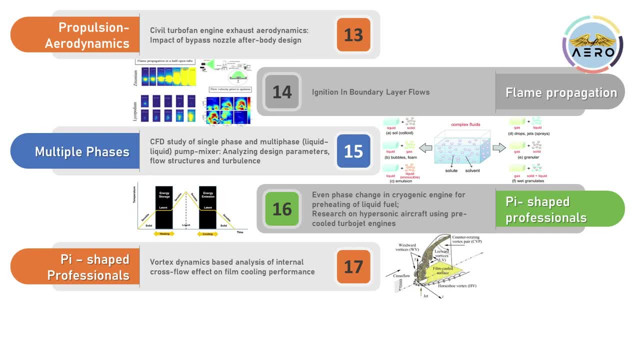 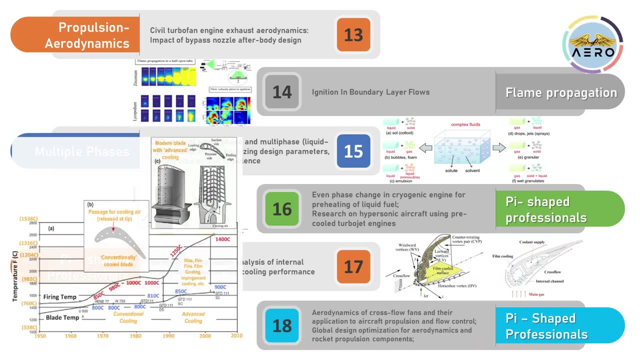 So talking about. one more interesting thing is a vortex dynamics based analysis of internal cross flow effect in a flint cooling- How the vortex dynamics plays an important role in a cooling. This is also one of the advanced research topic You can take up. 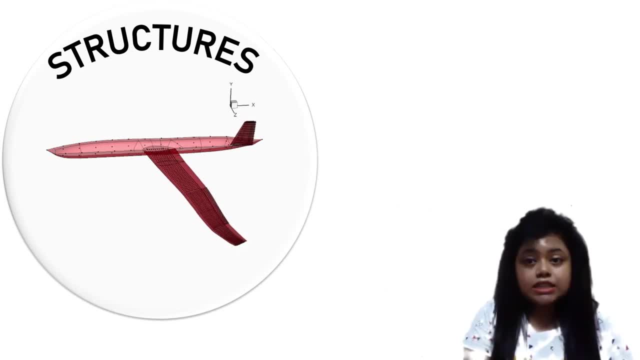 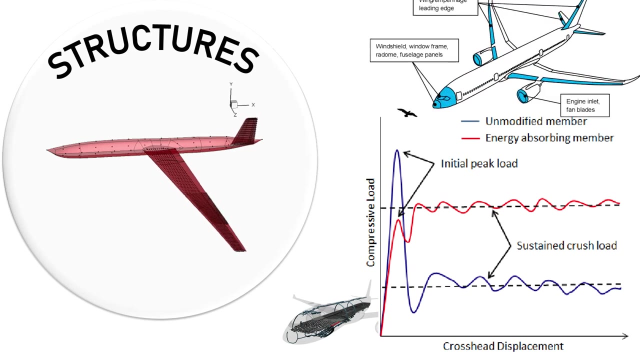 After propulsion, moving to an structured topic. So do not get confused with the materials. Materials I'll be explaining separately. So, talking about the research topic on structures alone, It is a vast topic and many wide domains. you can work on it or we can categorize into it. 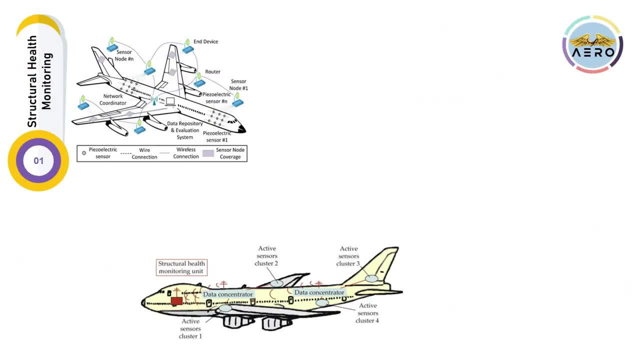 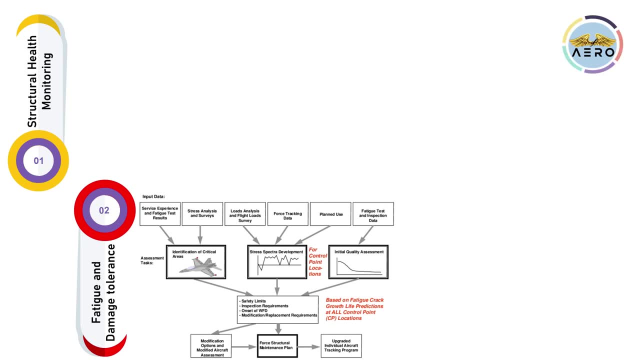 Like you can work on the structural health monitoring, Fatigue and damage tolerance of aircraft structures Or components or the parts of aircraft- Nut and bolts or whatever- Then morphing structures or multi-functional structures. Now, this topic is highly, highly working at present scenario. 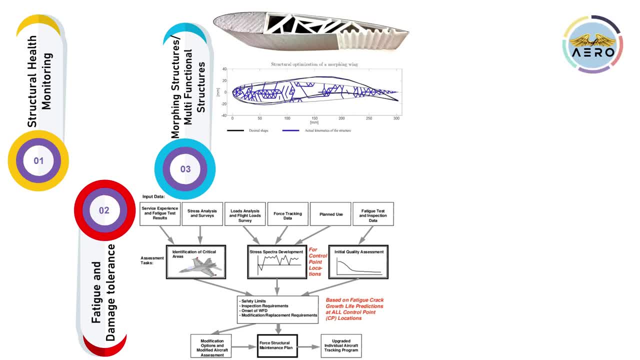 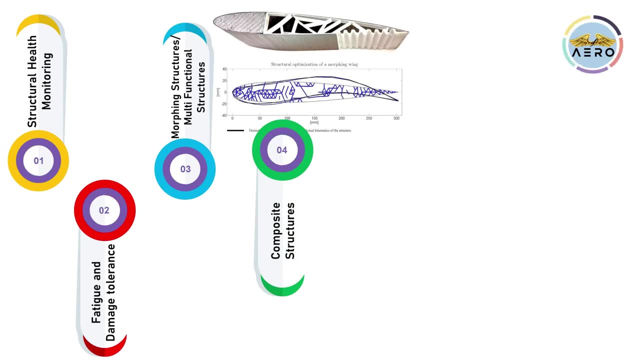 And I think this is the future. If you are specialized in structure, you must take up this topic and work on it Now. developing composite structures: This is also an another development. Another developing composite structures: I think this is also another very highly demanded topic. 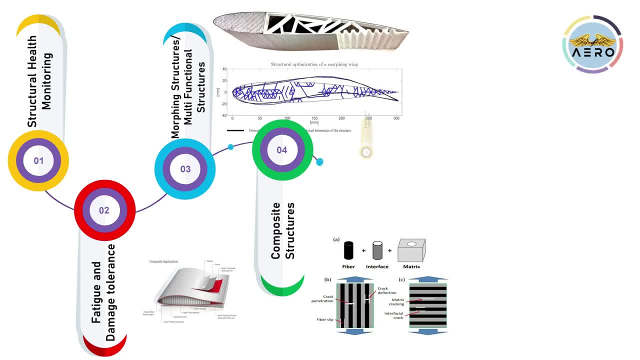 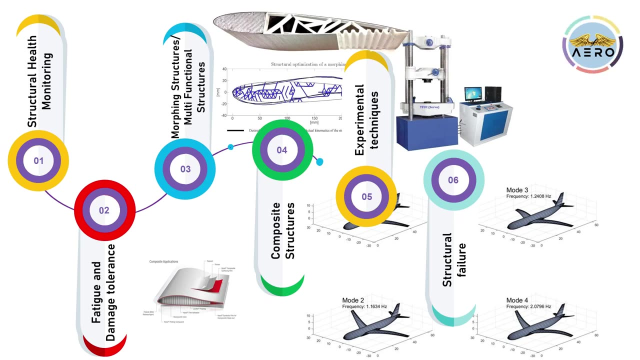 Then coming to us, experimental techniques to move the properties of structures, Our analyze of the structural failure, Then micro or nano finishing surfaces in multi-functional structures or in the general conventional structures. This also plays a very important role In that you can Add up one pie professional. 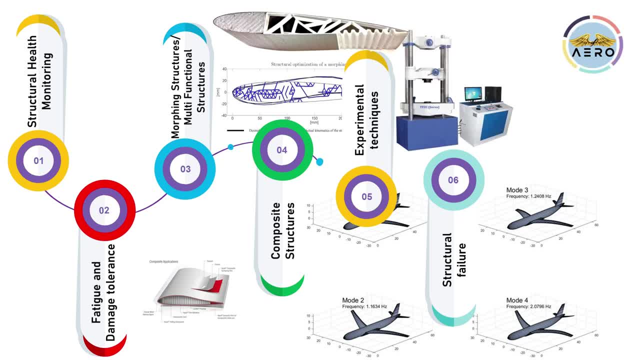 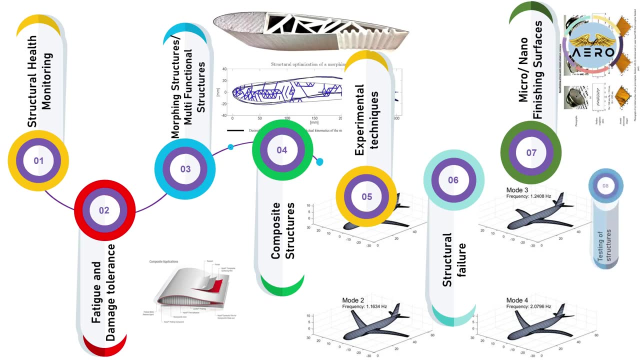 Like, you have one conventional one and you have made the same one with an 3D printing, And when you are making a finishing micro or the nano finishing, You can make a comparison data and you can bring up some research out of it. Then testing of structure through various entity techniques. 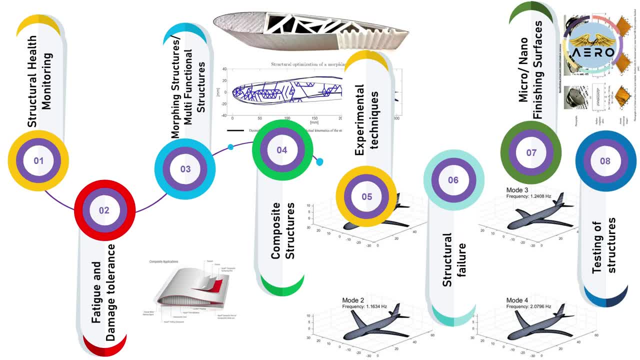 This also can be performed And let me tell you this: entity techniques are ample of entity techniques. You can take up one of the techniques and you can get the result. Keep in mind, in every case, You need to apply an adaptive finite element techniques and modeling tools. 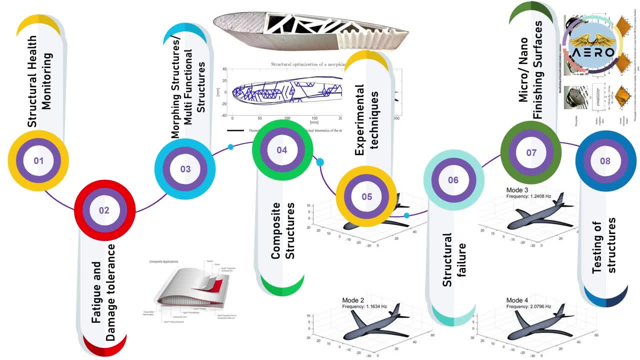 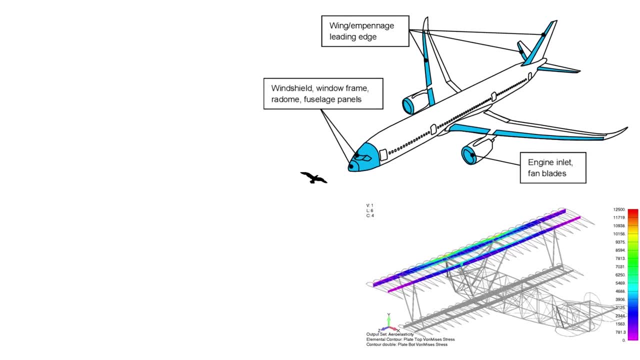 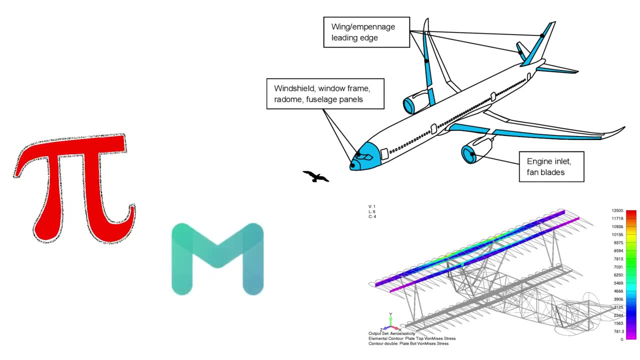 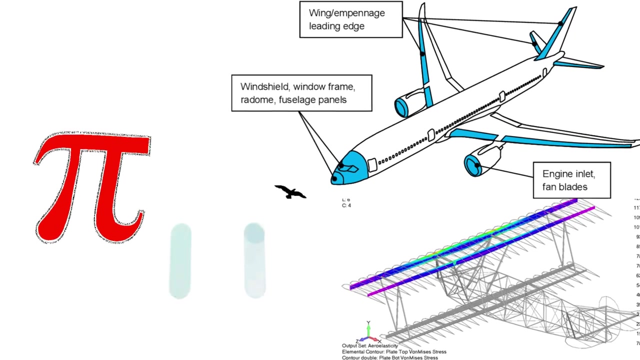 Or an experimental techniques to evaluate your results. Okay Now, considering today's research on structures, are more into an pie shaped or M shaped professionals, Where the research work with aerodynamics, Propulsion, Material Design, Manufacturing, Controlling, So all are combined together. 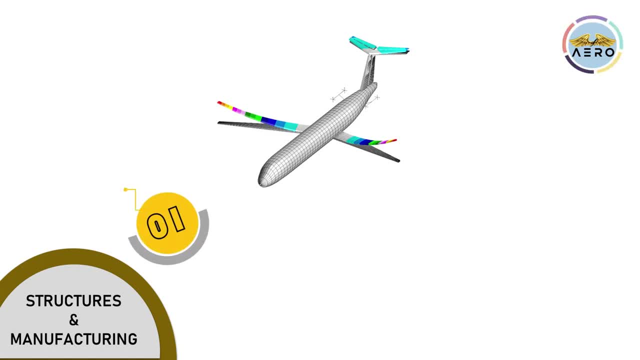 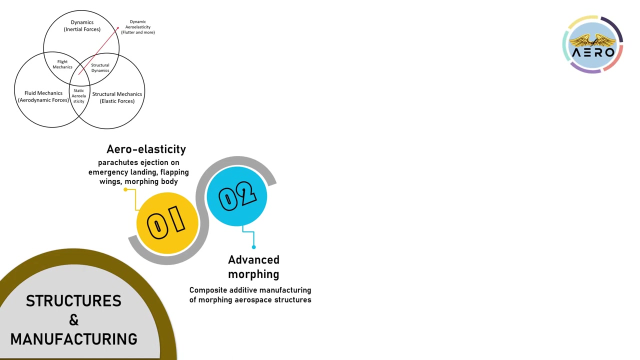 Let me highlight the more interesting and the present research progress or the nearing future. The oscillating airfoil dynamics play a key role of aeroelasticity topics, Even in morphing. some research has been undertaken, like Composite additive manufacturing of an morphing aerosite structures. 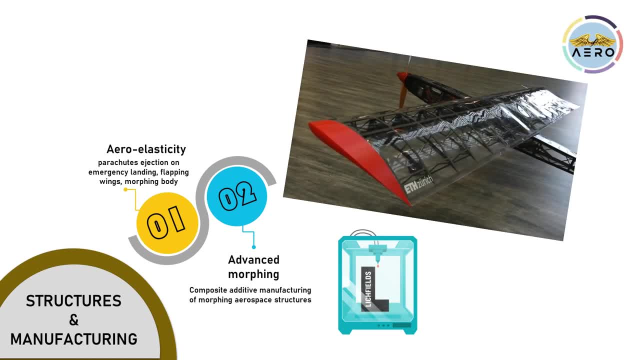 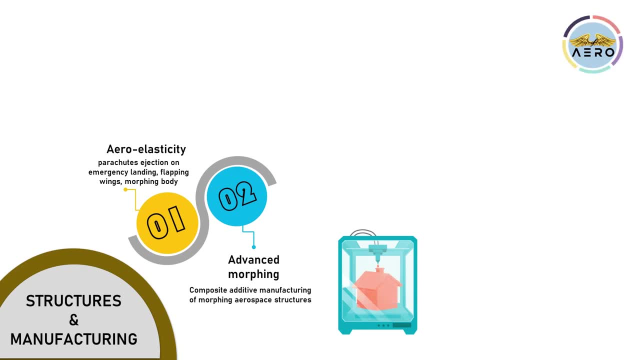 Okay, Talking about this additive manufacturing. Now, this is also one of the key role play in the structure group. This additive manufacturing structures, compared with a conventional one, Like 3D printing technology, has a wide scope to reduce the weight than a conventional manufacturing. 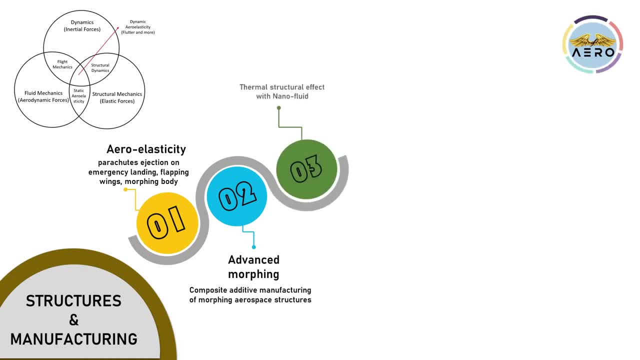 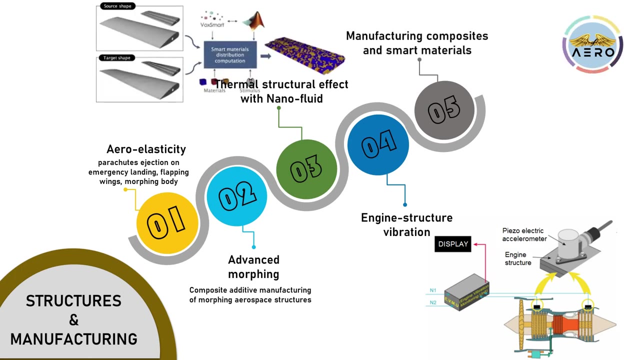 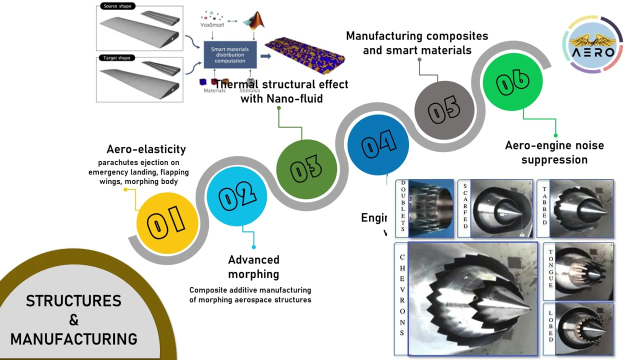 Then nano fluid for cooling thermal structure and its impact. Okay Now engine structure, vibration due to instability, combustion, Then manufacturing composites and smart materials and various type of processing. Then computational aero engine noise suppression. I have said like, there are couple of like, there is wide scope of opportunities to do research on this and pie professional. 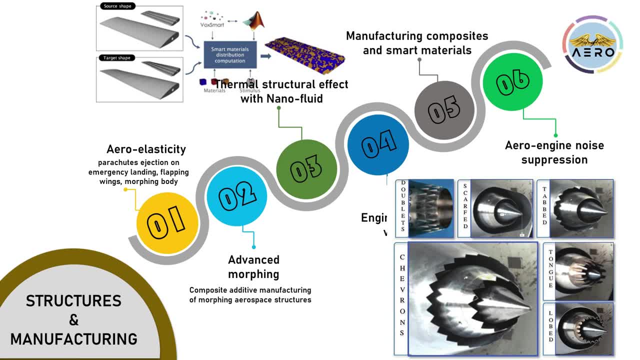 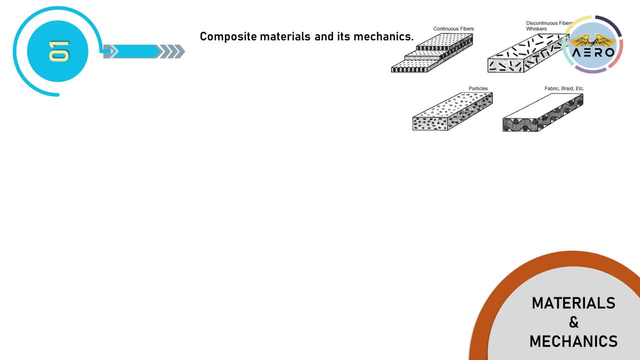 Then, talking about a correlated topic with a structure, is the aerospace material and the mechanisms. There are a wide variety of opportunities and the scope to work on, Like a composite material and its mechanisms. Now, talking about mechanism, There are various forms like computational mechanics, experimental mechanics, multiscale methods and the thermo mechanics. 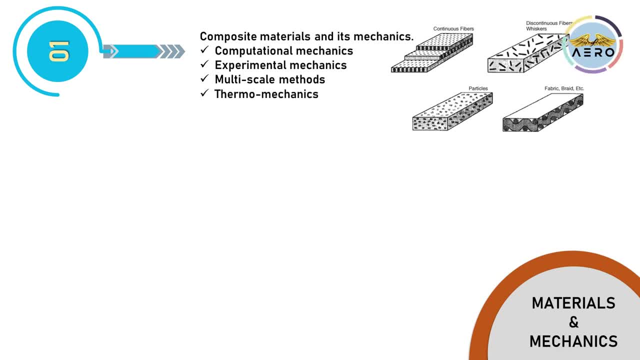 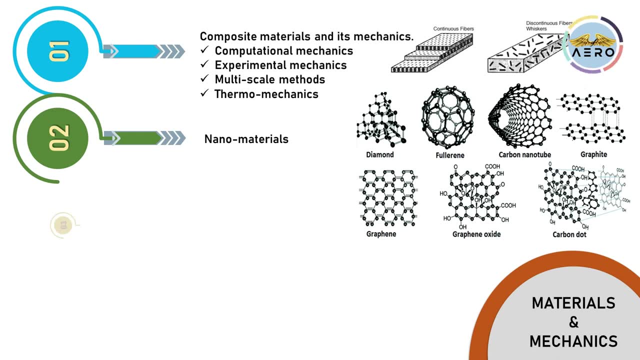 You can work on any sort of mechanics of a material. Now talking about next material is a nano material, Then high temperature material, Then alloys such as aluminum based alloys, the magnesium based alloys, titanium based alloys, nickel based alloys and ample of alloys you can work on. 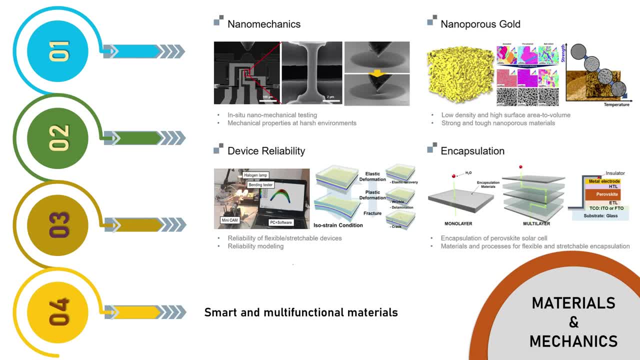 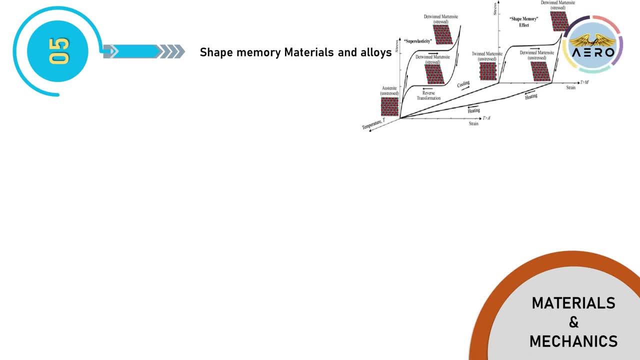 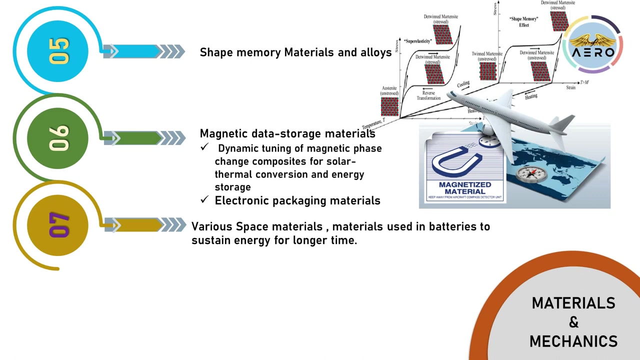 Then the smart and the multifunctional materials: Shape memory alloys and the materials. Then the magnetic data structures materials. Now this had a wide range of applications, or you can say a pie professionals. Similarly the electrical materials, Electronic packaging materials. Then there are some various space materials, like materials using battery to sustain energy for a longer period of time. 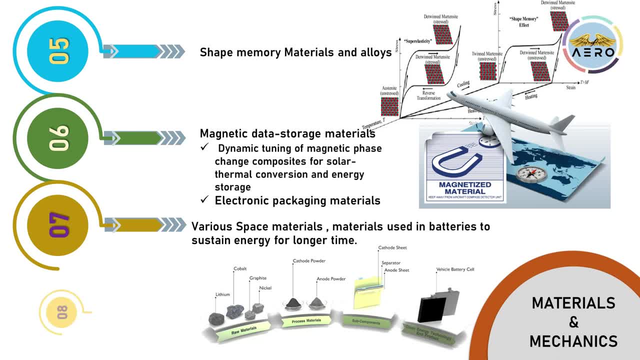 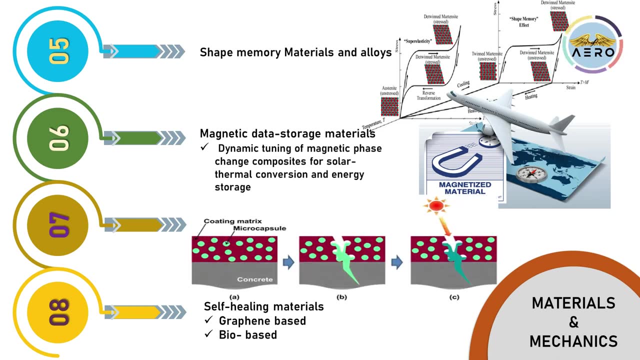 One more very special and unique work you can do is a self-healing material. Now, at present we are also doing a graphite base, But nowadays some more researchers are working on the bio based self-healing material, Because the fossil field resources are going to get exhausted or the oil price gonna rise. 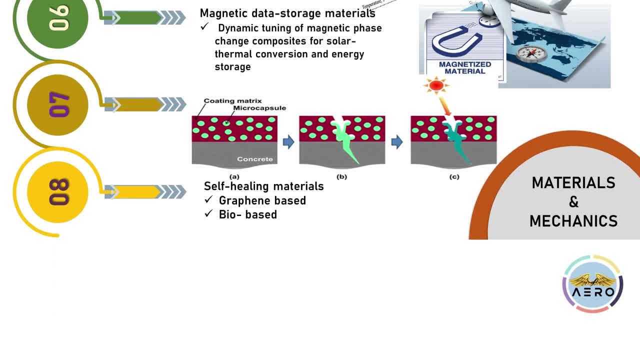 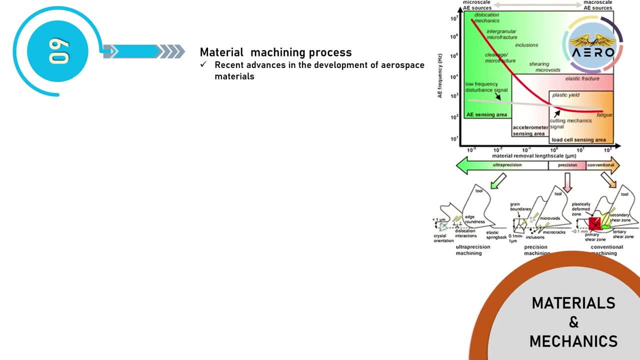 Now upcoming research is in bio based self-healing material. Then a material machining processes, especially. there are lot many types or the recent advanced in the development of the aerospace material you can work on. Then one more thing: a special material coating. Special material coating for the thermal insulation or the effective cooling. 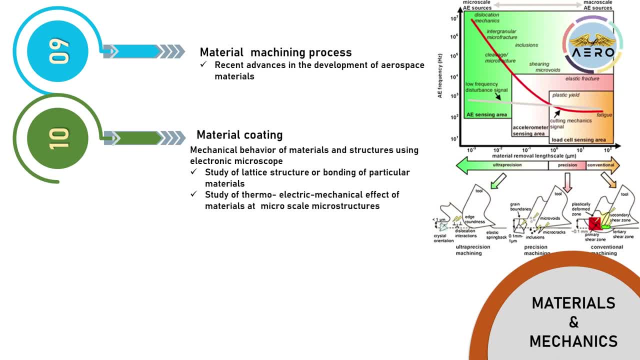 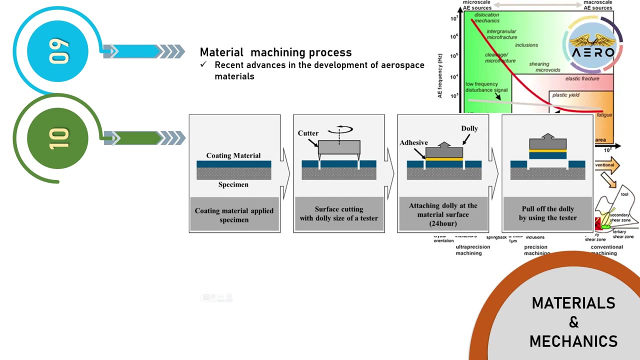 Now, then, also wide many opportunities like to find out the mechanical behavior of an unique materials and the structure using an electronic microscope. Then study of a lattice structure or a bonding of particular materials, Study about thermoelectrical mechanical effects of material at an micro scale, microstructures. 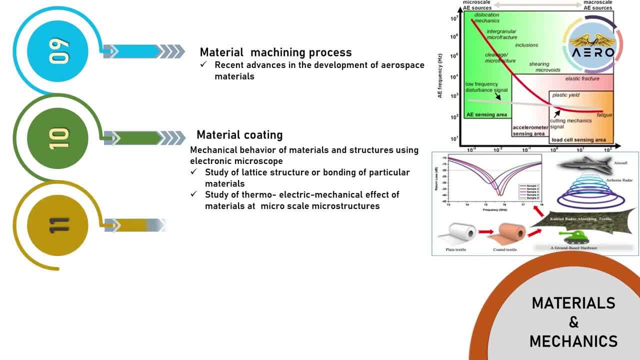 Okay Now. study effect of metamaterials on an atom. Okay, Okay Now. study of a radio acoustic properties Like an radar absorbing material. All of you might be knowing most of the aerospace. people will be knowing what is and where this radar absorbing material is used. 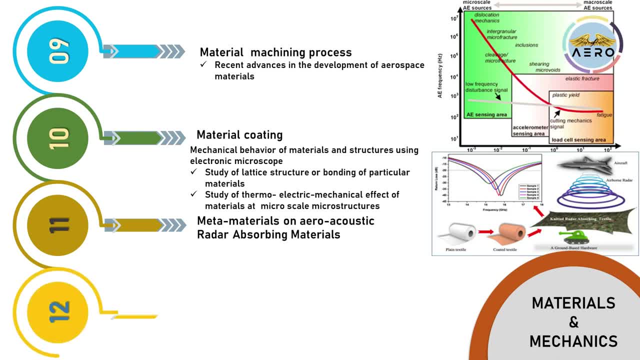 Called as a RAM material sometimes. Okay, Then multifunctional material systems to control the shock, vibration and the sound, like a damping assessment of a new functional materials, aerospace materials, Which is comes under the pie shaped research profession. Then bending mechanism for morphing aerospace applications. 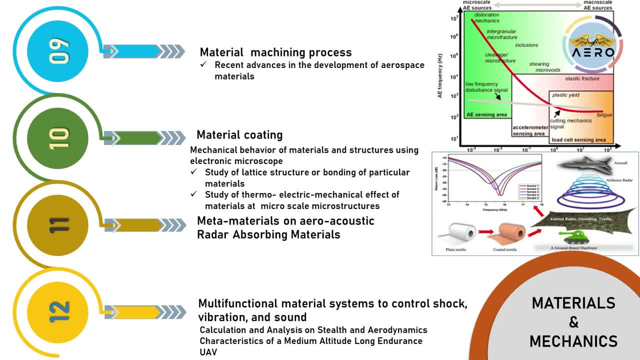 Then calculation and analysis of stealth and aerodynamic characteristics of various aircraft or the structures. This also play a very important or a key role in this, also a type of a pie pie shaped professional, Where both the design knowledge is required, Aerodynamics is required. 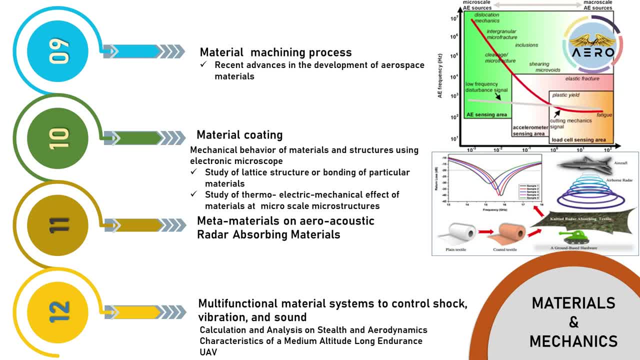 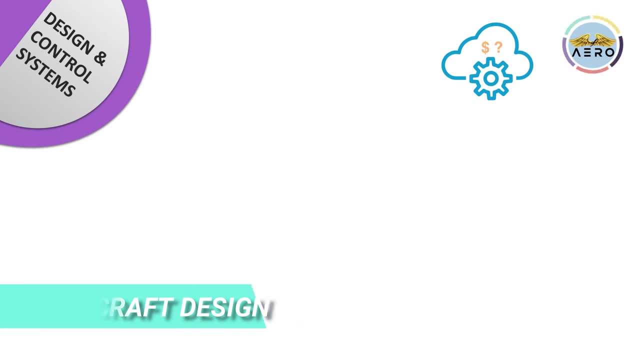 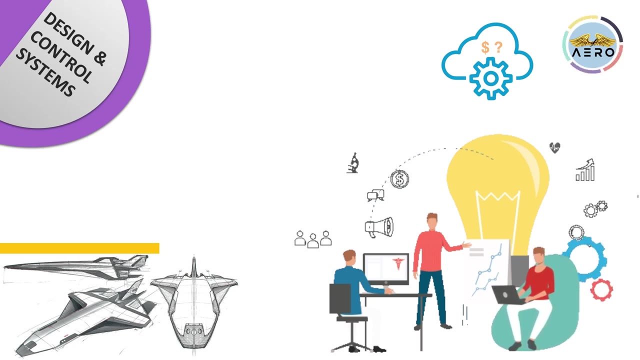 Propulsion and the material: Okay. Now, after aerodynamics, propulsion, structure and materials, comes the design. Okay, And it is a multidisciplinary domain which comes under the pie shape professional or an M shaped professional, Because here we need to know her idea about a computation and analysis, numerical methods where it need to transform and give an impact, a new way of design. 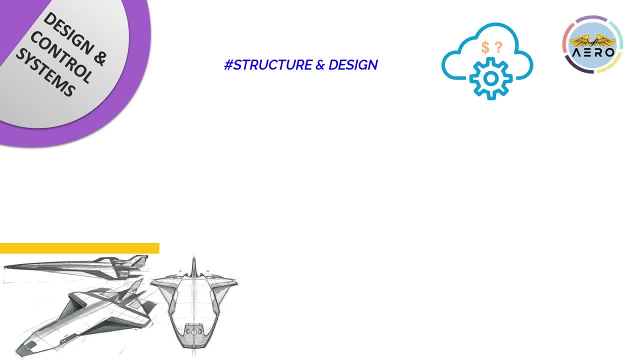 Okay, And sometimes it is been combined with the structure and design or the design and manufacturing or the design and controlling. accordingly, I have been categorized into four forms. in cognition and the design theory, It is applicable for an modeling of any aircrafts or aircrafts or UAVs or airplanes or any mission analysis for a novel aircraft technologies. 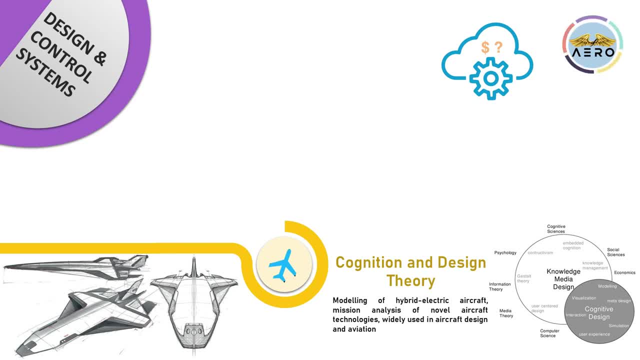 Like mostly used in aircraft manufacturing, Okay, And then also used in aircraft designs and aviation in drasties. Now, talking about a design automation, It is applied to an aircraft modeling and optimization of any aircrafts: UAVs, Drone- Now, basically, what is drone? 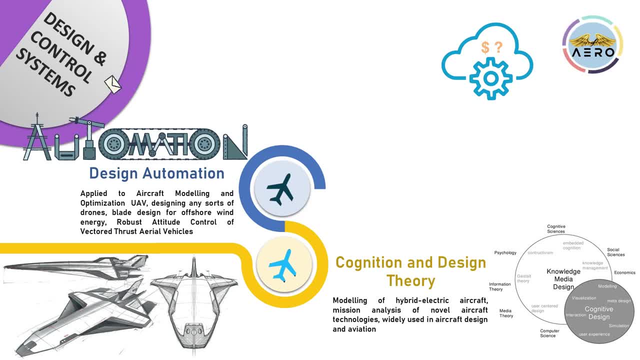 Drone is a dynamic, remotely operated navigation equipment. Now, here also, when we talk about navigation, It is a both. we need a knowledge of a design as well as a controlling. then artificial intelligence and the robotics will be play a key role in this design automations. 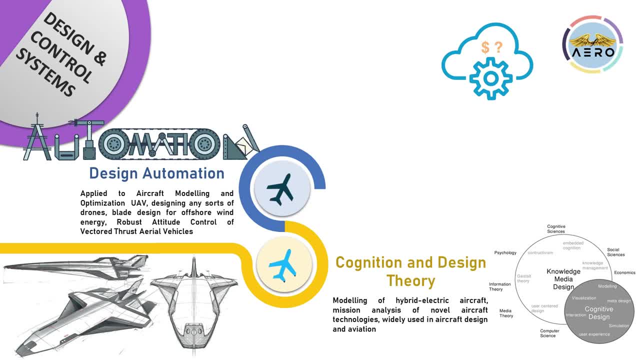 now talking about um sustainable design, an efficient engine design for an fuel efficiency or compatible for a biofuel system. such kind of design can be seen as a sustainable design. now you can also work on recent uh recent advances in the fuel sale based on the propulsion system for an uav- or mostly it is using uav- that ample of research can be done on sustainable. 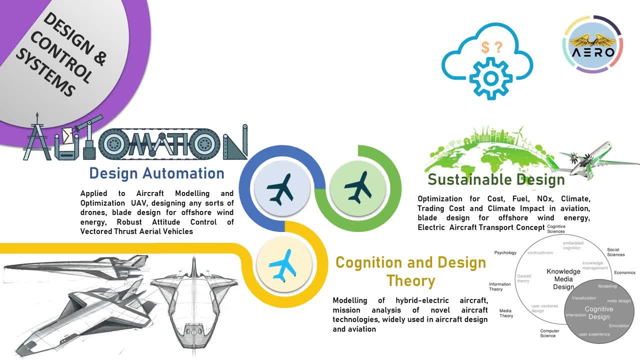 design. now coming to an complex uh system design. this can be of the robotic arms, or maybe a landing gear mechanisms or any other mechanisms: fuel tank design, landing gear systems, aircraft systems, maybe hydraulic pneumatic. such kind of designs will fall under this complex system design. okay, now 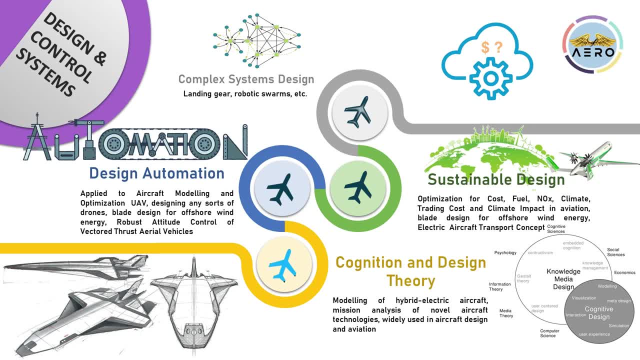 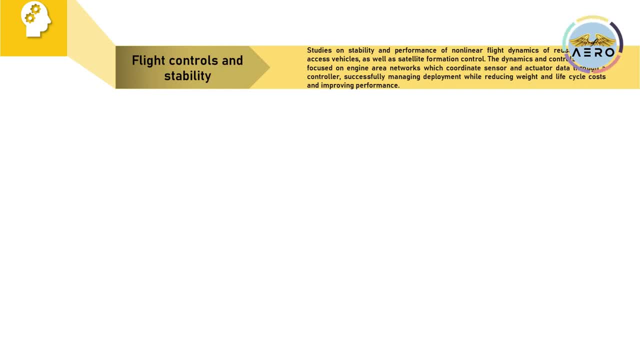 looking close into another important field of control system alone in aerospace, where you can choose a strong multidisciplinary system- oriented that emphasis- a linear and non-linear system okay, and where also optimization, feedback, control, optimal planning and decision making. then stodiacast stick process, software aspects of flight systems. now one must evaluate the computational and 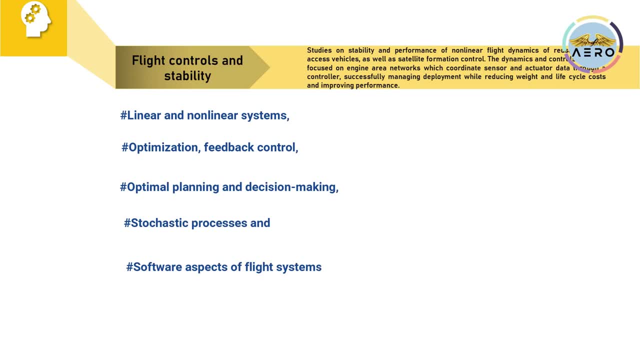 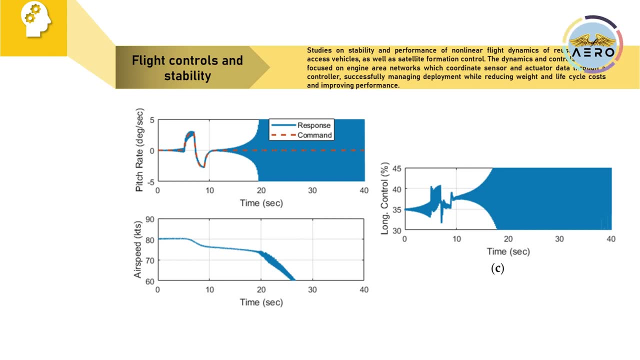 mathematical approaches through matlab and the python in the most of the cases. okay, now looking here, this control system. here, first of all, the flight controls and the stability, or study on the stability and the performance of a linear and non-linear flight dynamics can be also involved in this topic. 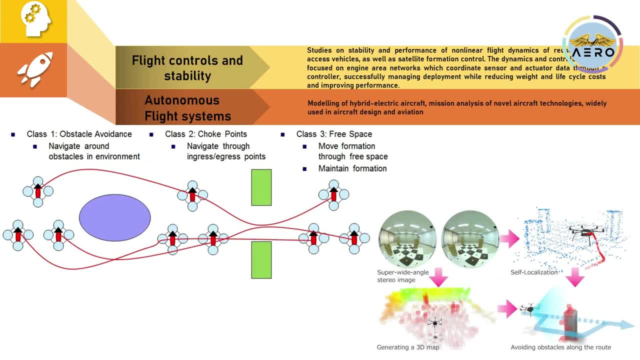 then talking about the autonomous flight systems. avionics systems include space robots, multi modeling sensors, then uh planning- uh, it may be a structured or unstructured- on uncertain uh structured avionics systems where you can maximize the information extraction from the sensor data and you can accordingly make the decision and predict and monitor the health of this avionics system. 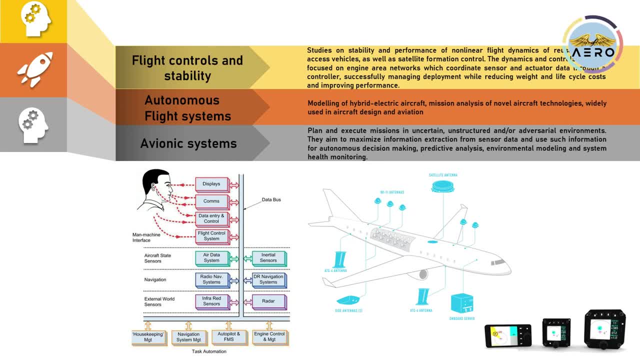 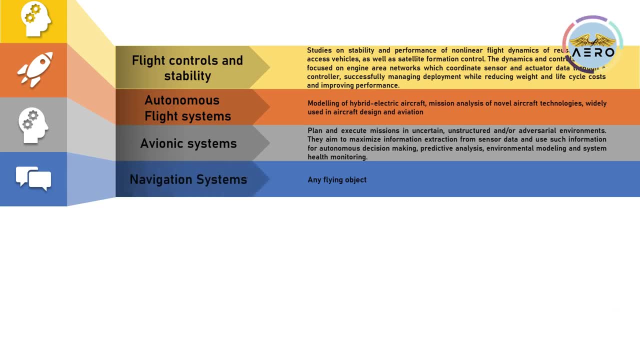 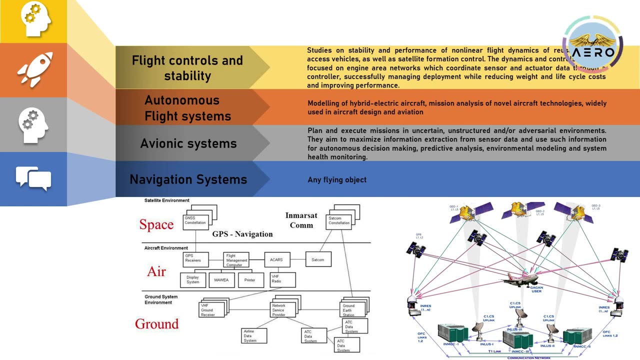 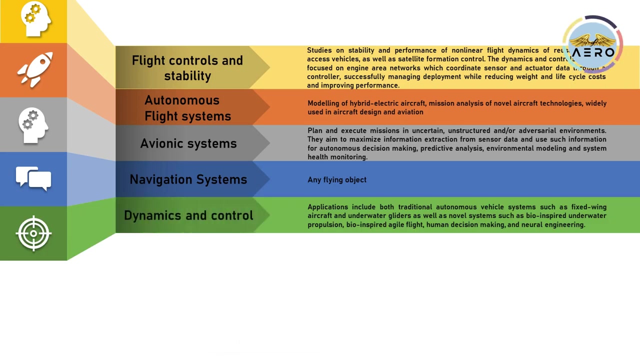 there are a lot many work you can do on this avionics system. then, talking about the navigation system to a navigation system, to any flying objects, talking from airplane, helicopter, uh, even missiles- then instrumentation. instrumentation is also a player, wide rule on this research field. then dynamics and control, often manned as well as unmanned air vehicle. there, 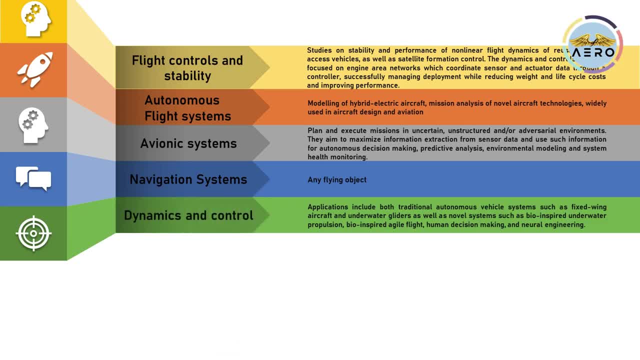 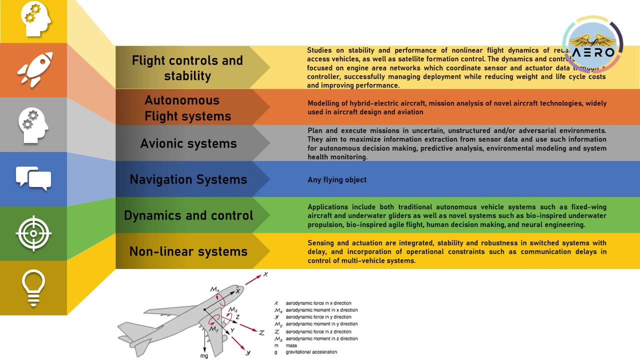 is a ample of research work. now i want to highlight a special category is a non-linear system where it happens, uh, where a wide variety of research can be done, like sensing and automation are integrated, where the stability and robustness is also switched to a new system, right. 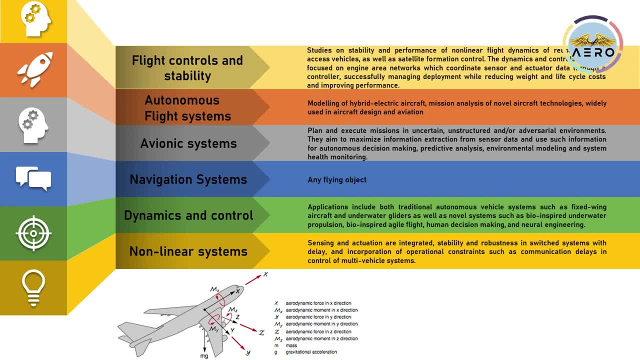 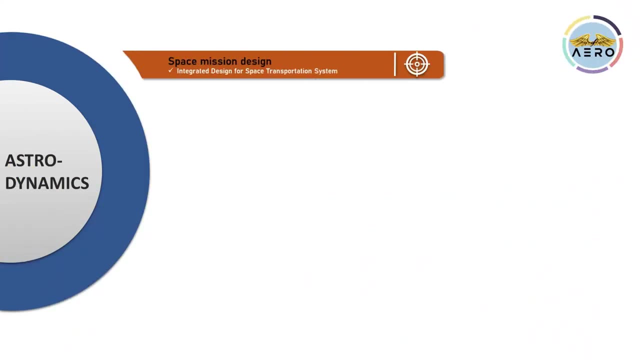 so this kind of work can be done and additionally, uh, this kind of applications you can also involve, like automation, vehicle systems, maybe of fixed wing aircraft, or underwater gliders or human flights and many more. then, as i've said, a few aerospace students can also enter to an another specific topic, like astrodynamics or the orbital. 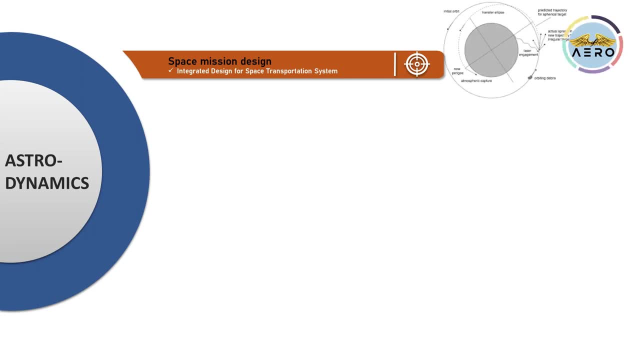 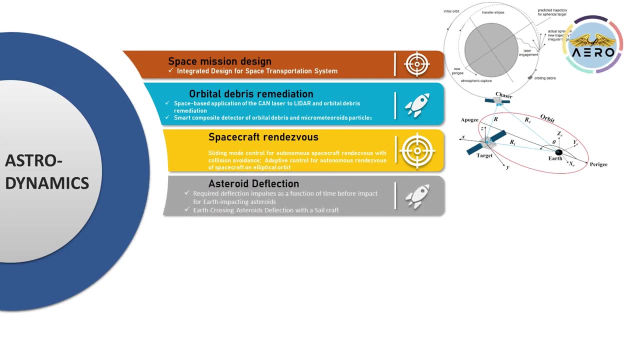 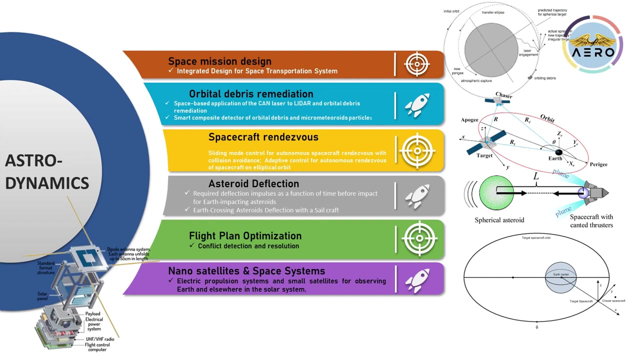 mechanics like space mission design, orbital debris in spacecraft- and this approximately operators- asteroid deflection, flight plan operations, conflict detection and the resolution of nanosatellites and the space system. talking about the space system, you can also work on the electrical propulsion system and making some small 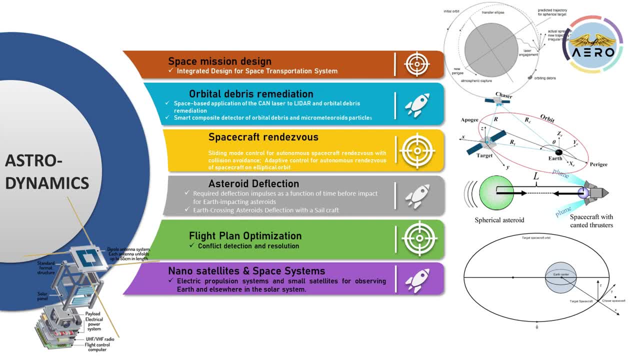 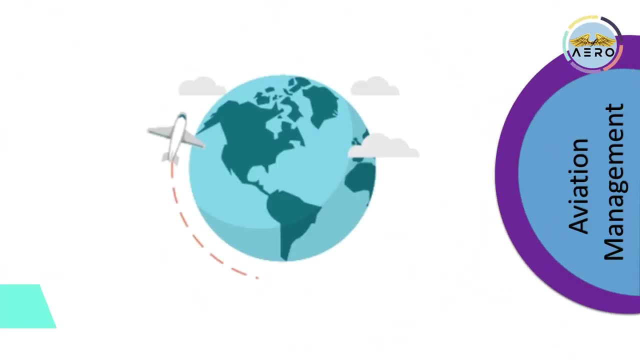 satellites for observing the earth and other uh whatever like in the solar system. so this all mostly comes under the pie ship. professional are adopted, then um, coming to us next is our aviation management. now possible research openings in the aviation management. so here also mostly very few uh students or do. 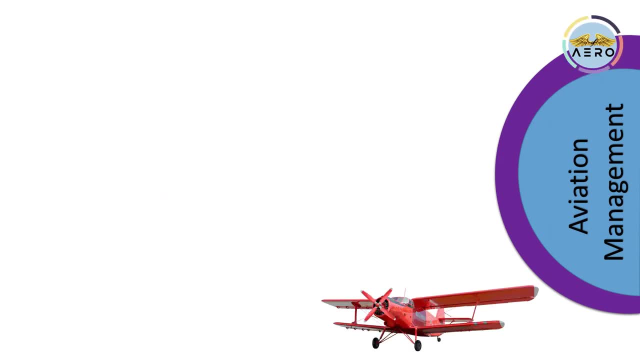 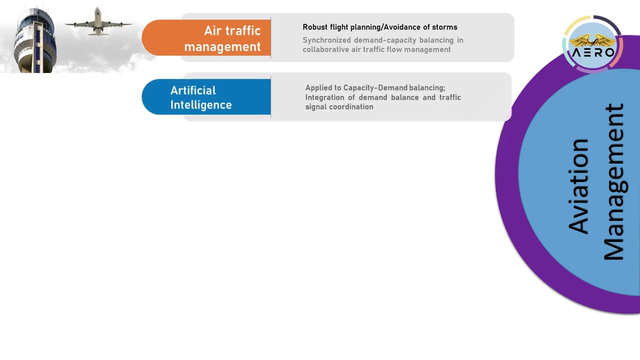 research on such kind of topics. so let us discuss that: what kind of topics we can cover in this aviation management. like you can do a research topic on the robust flight planning or air traffic management, then how to make an air traffic management in the by avoiding of storms, okay, 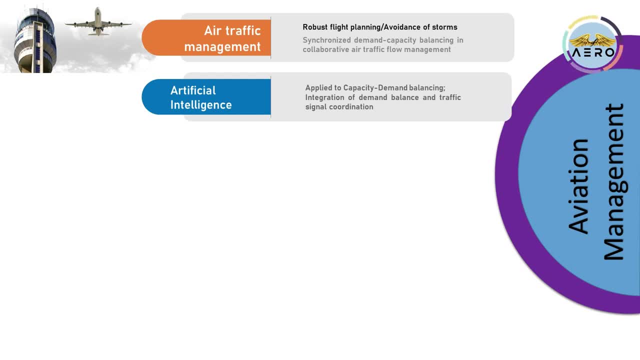 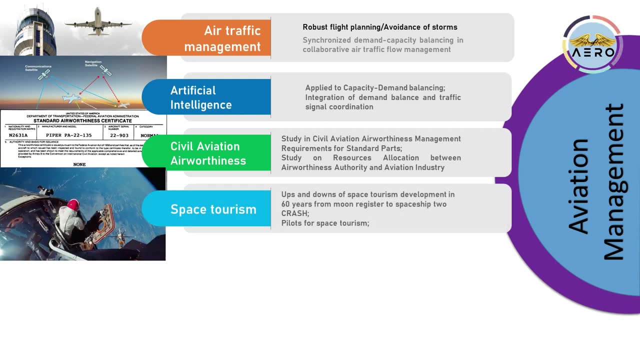 artificial intelligence applied in the capacity, demand balancing, civil aviation, air wilderness management, space tourism service logistics and maintenance management, then supply chain and the air transport management or even the aircraft manufacturing logistics you can work on. uh very interestingly, recently uh i have been great and amazing uh research topic on integrating air and 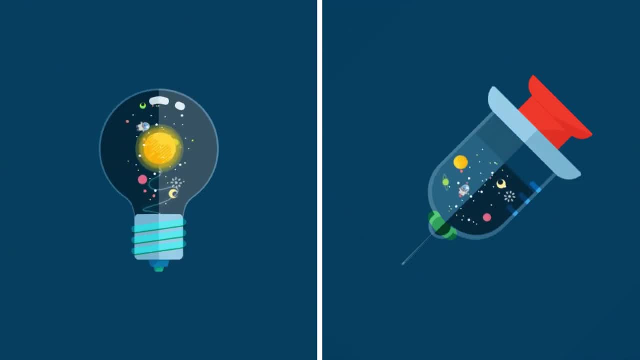 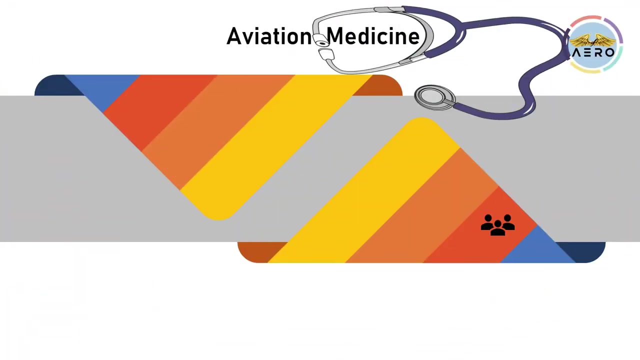 nearing space, traffic management for aviation and nearing space, if you are like, even some more research in air and space laws. but uh, that's are for the legal people, not for the engineers looking into the aviation or the aerospace medicine research. it is not for core aerospace engineering work but mostly mbbs people are, or the doctorate are doing, working on the such topics. 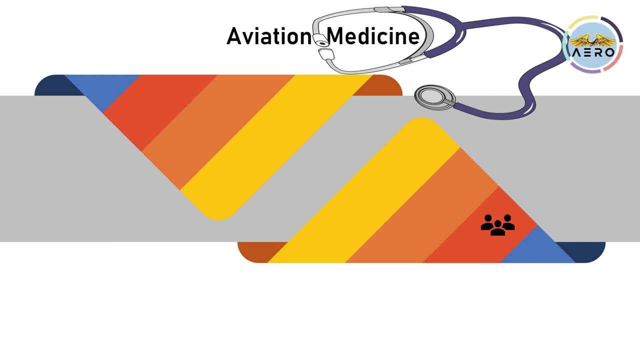 and it seems to me quite interesting. so i thought uh, i can share a pinch of idea about this. uh, space medicines, like uh there's some more work has been done, like um aeromedical solutions for aerospace safety, then aviation medicines- how the illness and the limitations for the flyers. 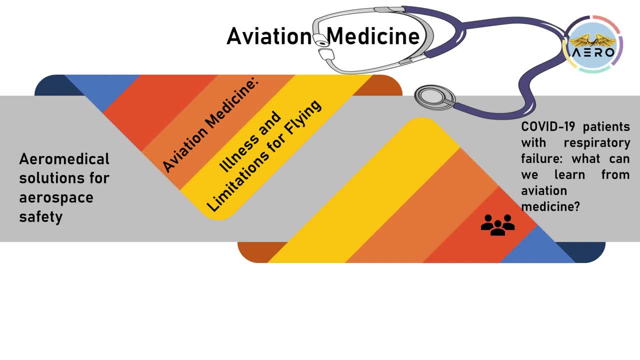 then, uh, at present, um, we are into 2020. now, covid 19 is going on. like in this also, i have a lot of further research that is being done on the subject of the simulation of the navigation on the flyers. then, at present, um, we are in 2020. now, covid 19 is going on. like in this also, i have a lot of research. 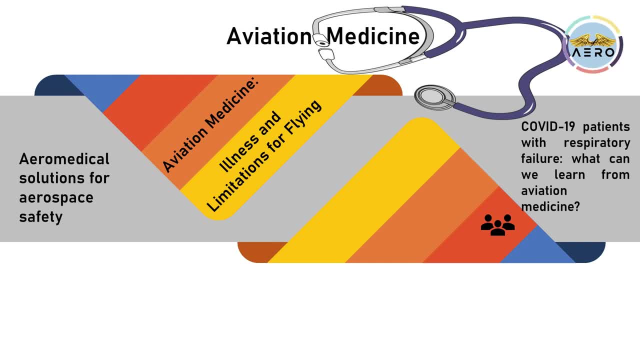 about flight administration and the device management policy and the things that we need to do. uh, we are doing, uh, more research on the specific값s, which is the project for aviation medicine, so we will be doing this. have read an article like COVID-19: patients with a respiratory failure: what we can learn from the